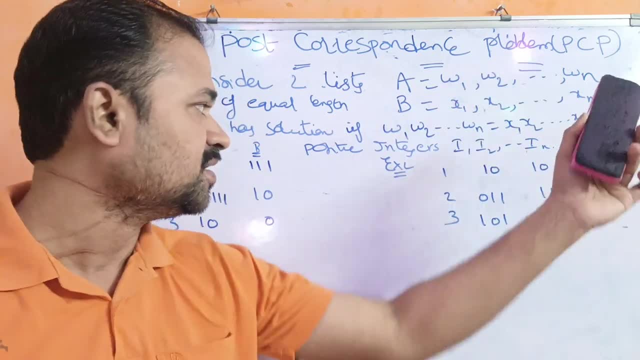 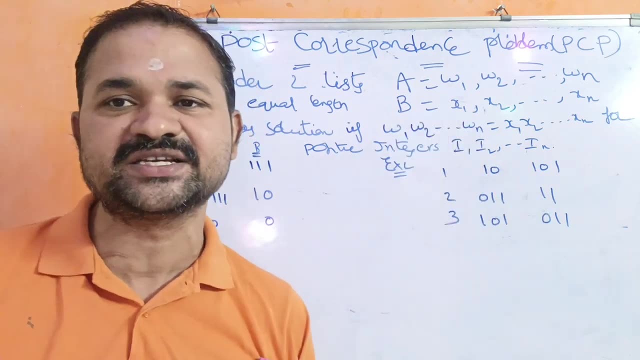 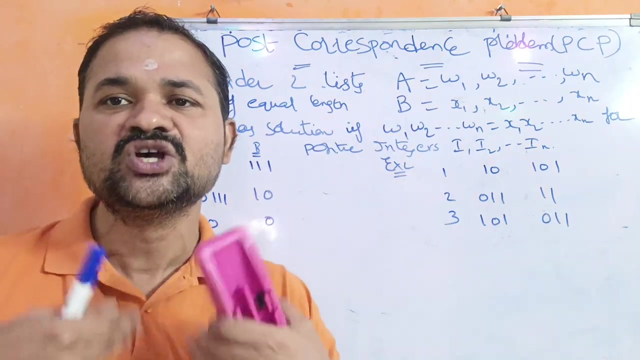 by concatenating x1, x2, so on, xn for all positive integers i1 comma, i2, so on in. so that means here these are the positive integers one, two, three, four likewise. so here we have two problems. so let us check whether these two problems has solution or not. let us see the first problem. 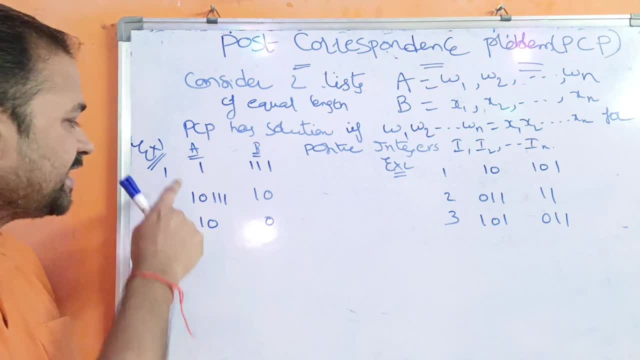 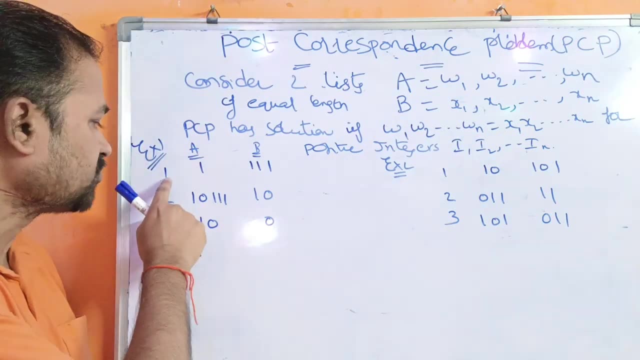 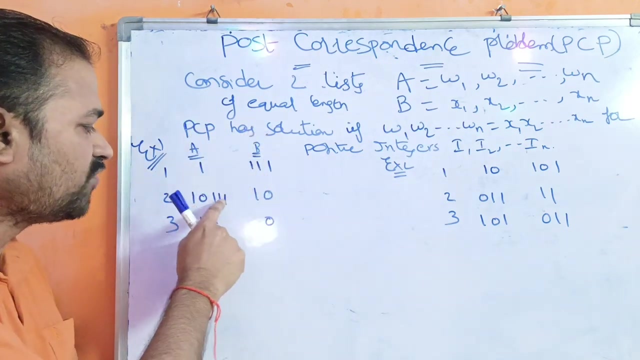 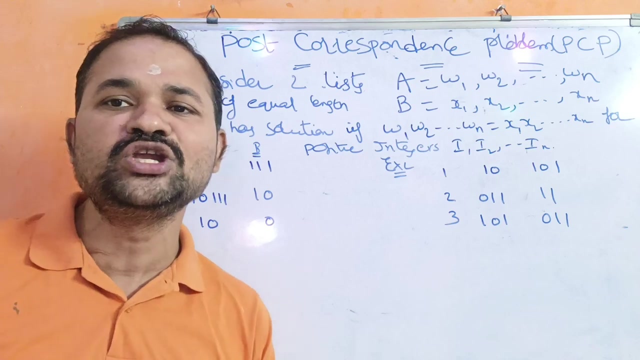 here we have two lists, a and b, and each list contains three strings, three integers, so one. so if it contains one, triple one, so this is a list, this is b list, so one, three will be one zero, three. one, one zero, one, zero, zero. so now we have to check whether this problem has solution or 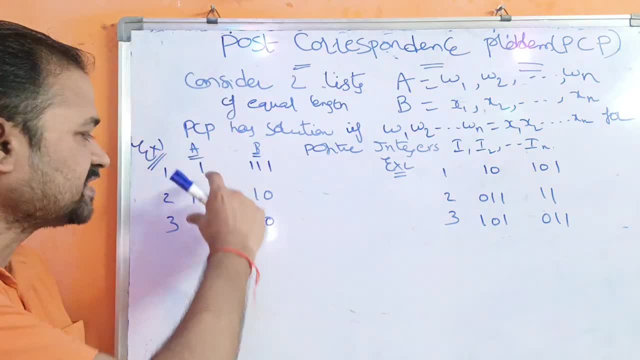 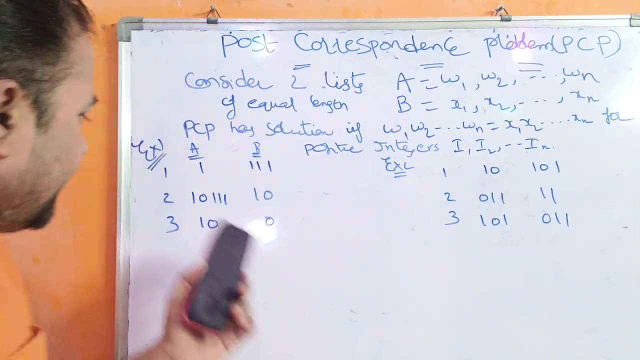 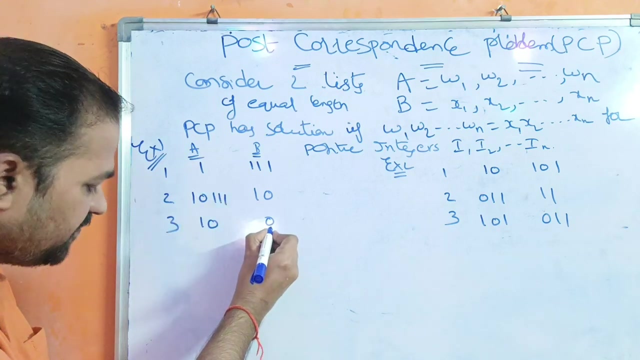 not okay. so that means the string, the strings formed by a must be equal to the strings formed by b. so let us, let us see here, so if we, if we observe the strings, we can see the problem here. strings here: Here, in A, we have 1, 0.. In B, here we have 0. So 1, 0, 1, 0. So these 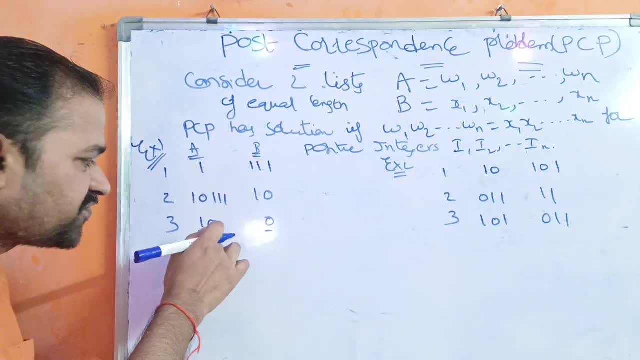 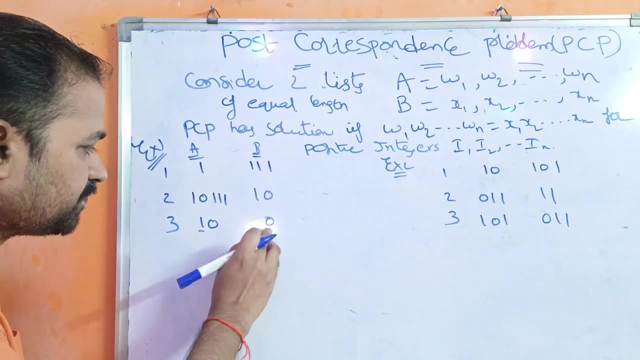 two are not equal. Why? Because here the strings formed by A must be equal to the strings formed by B, But here the first character is different, So we cannot take this one. Next, here the first character is 1.. Here the first character is 1. So both are same. So we can take this. 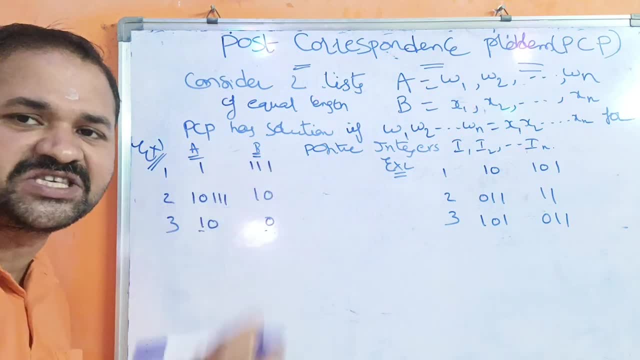 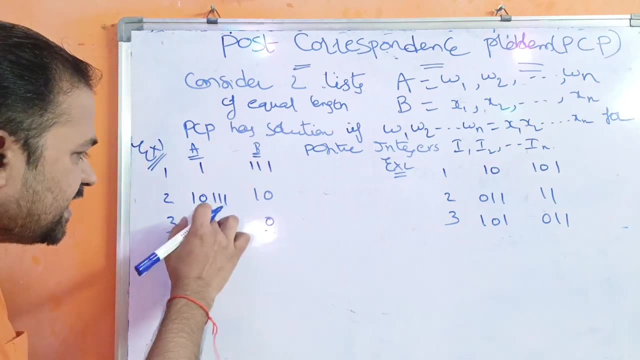 one Here: 1, 0.. Here 1, 0.. We can take this one. So here this problem has multiple solutions. Here our target is: we need to find one solution. So let us take the second. 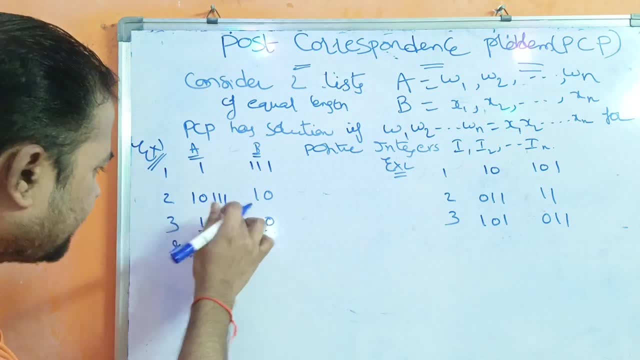 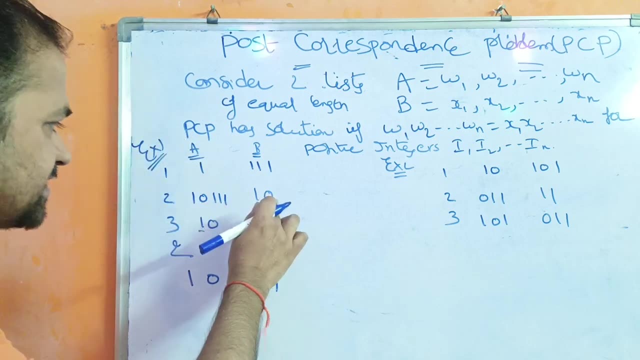 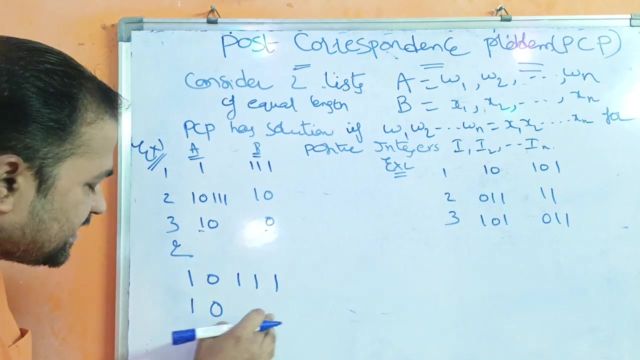 one, So 2, 2.. So what is the string here? 1, 0, 1, 0, 3, 2, 1.. Next, here the string is in B. the string is 1, 0, 1, 0.. So next we have to select a string in the. 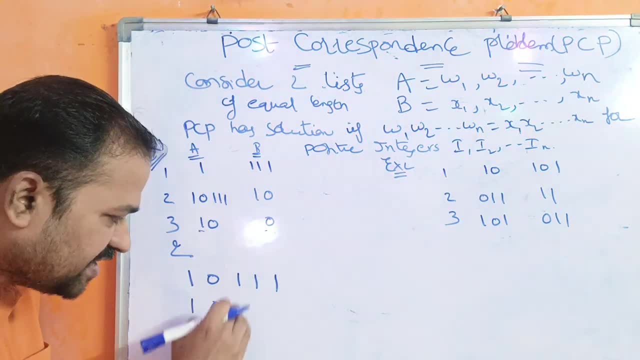 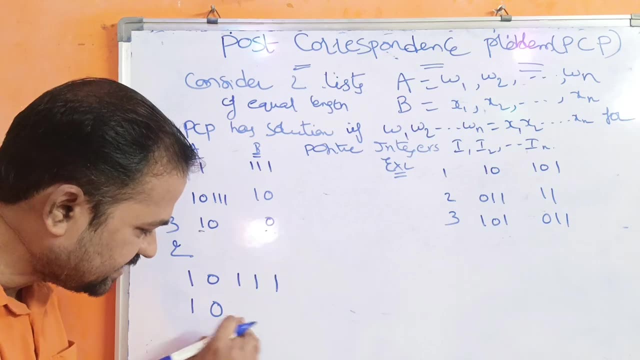 B In such a way that it should start from 1.. Why? Because here what is the third character, 1.. So we have to select the string in such a way that it should start from 1.. So let 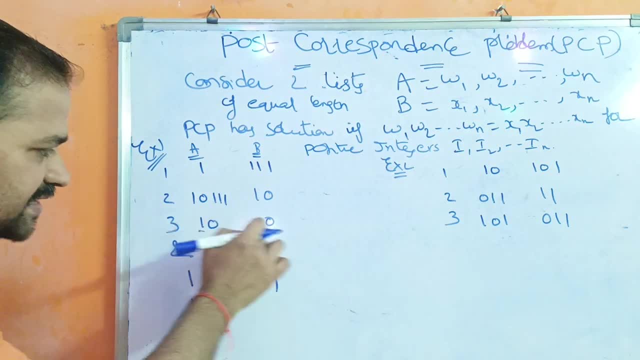 us check here. So it starts with 3.. We can't take 3 here. Why? Because here the string is starting with 0. So can we take 2?? We can't take 2 also. Why? Because, if we take, 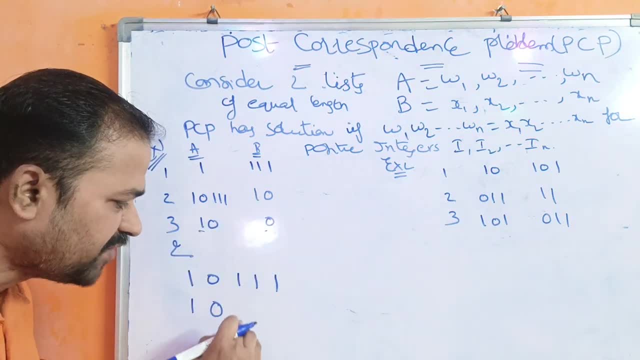 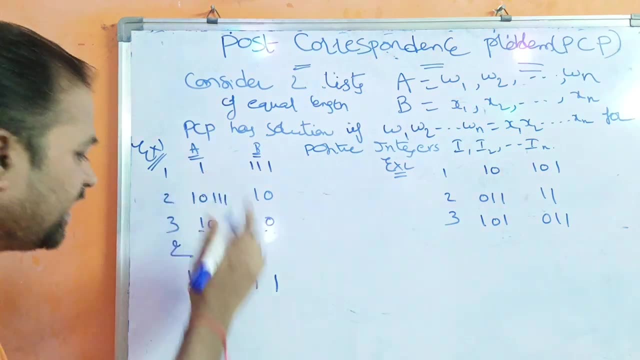 1, 0,, then we will get 1, 0.. So 1, 1,, 1, 0.. These two are not equal, So here the choice is only 1.. So the next sequence is 1.. So in A the string is 1.. In B the string is 3, 1.. In B the string. 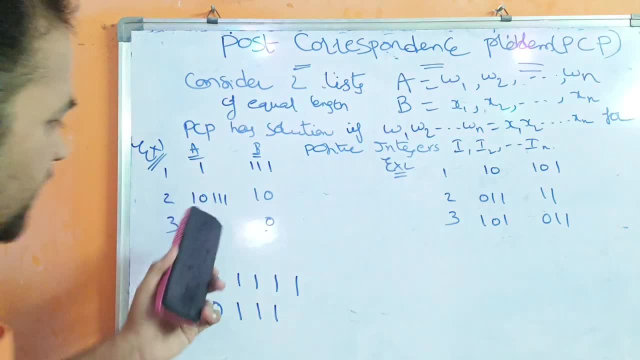 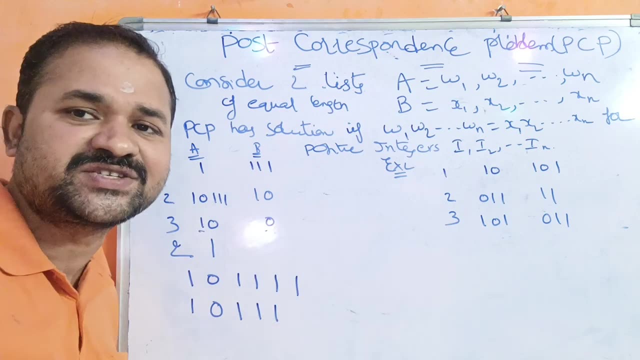 is 3, 1.. Okay, In B the string is 3, 1.. Here we can take a number more than 1 also. So we can take the string 1, more than 1 also. There is no problem. But we have to. 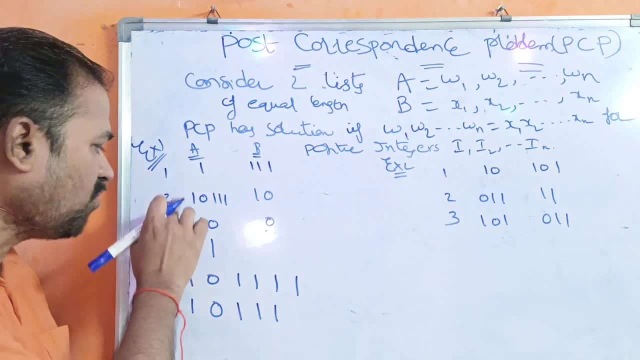 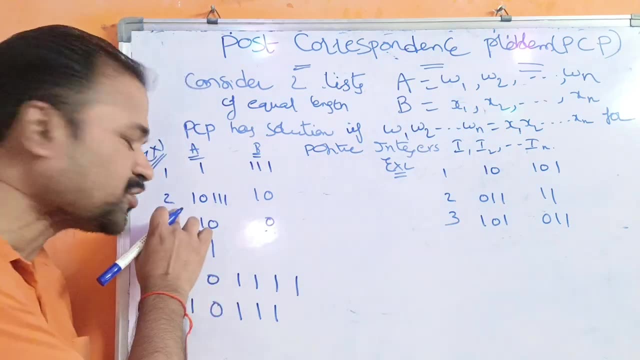 cover the three strings Here. we have 1,, 2, 3.. We have to cover 1,, 2, 3.. It is our choice. We can repeat a string more than 1 also, So we can repeat 2,, 3 times, 5 times or 4 times also. There is no problem. Okay, So let us. 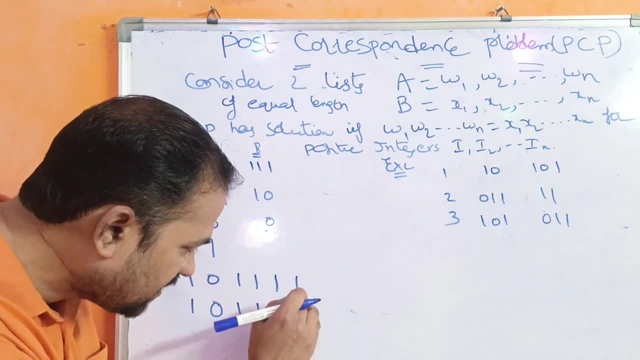 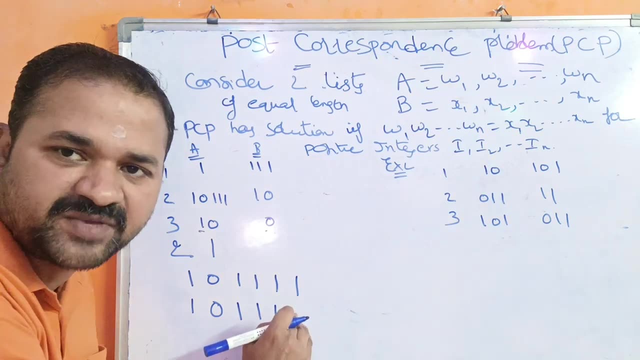 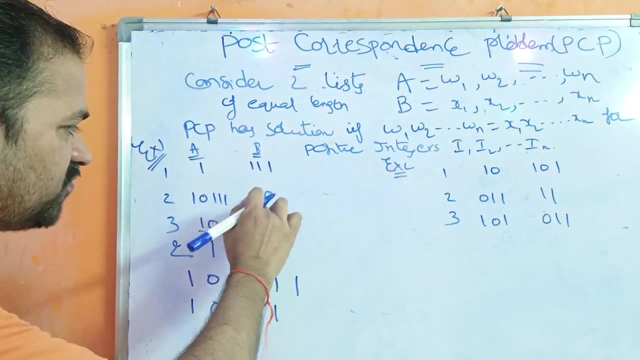 consider the next one Here. what is the character here? 1 here. So we have to select a string in such a way that it should start with B. It should start with 1 in B string. So if we consider here: here we have 3, 1, 1, 1, 0, 0. 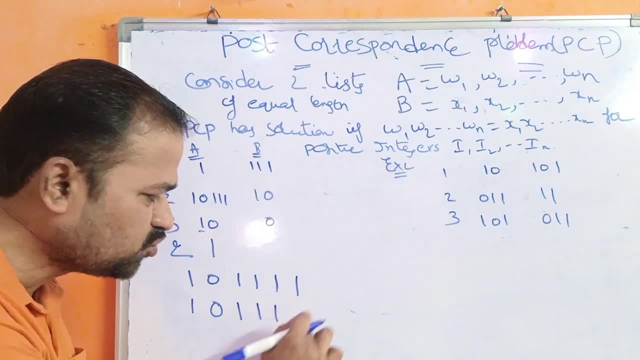 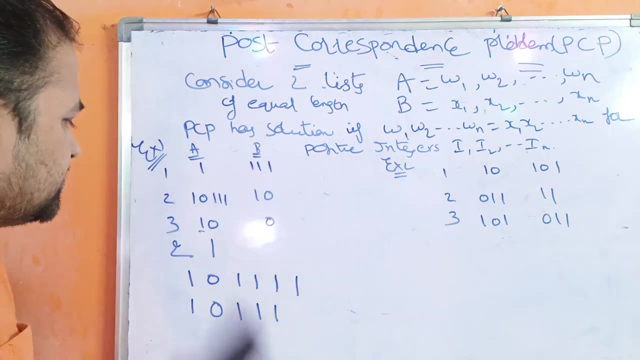 We cannot take 0 here. Why? Because if we take 0,, then these two are not equal. So we can take either 1, 0 or 3, 1, 1 also. Okay, So it is silent error approach. Let us consider: 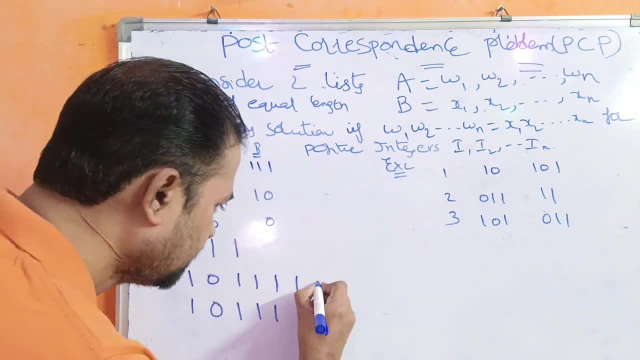 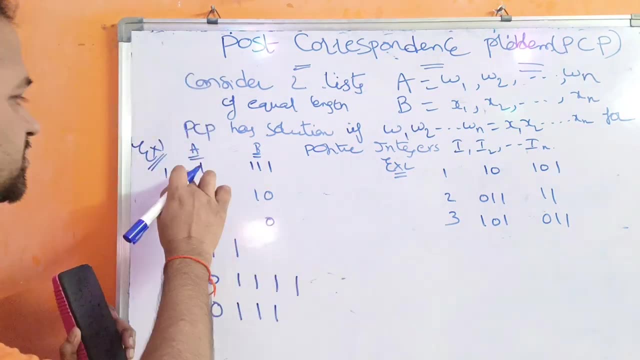 1 here. So 1 means here 3, 1, 1.. 3, 1, 1.. Next, I am sorry. So 1 means what is the string 1? is the string 1, is the string Variance. here we have to take 3, 1,, 1.. 3,. 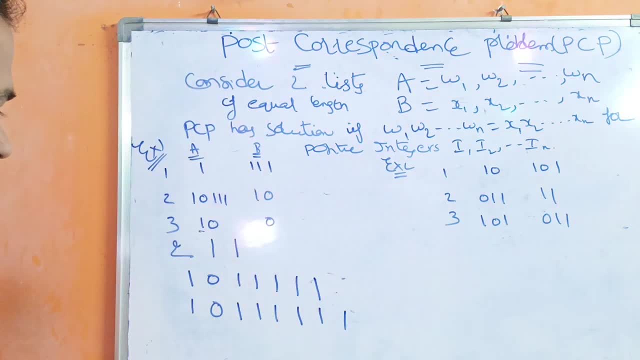 1, 1.. In B we have 3, 1, 1.. So we have 3, 1, 1.. So next we have to consider a string in such a way that it should start with 1.. It should start with 1.. So we can take 3 here. We can take 3 here. Why? 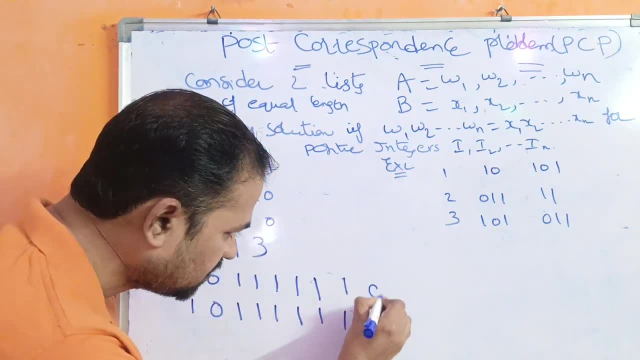 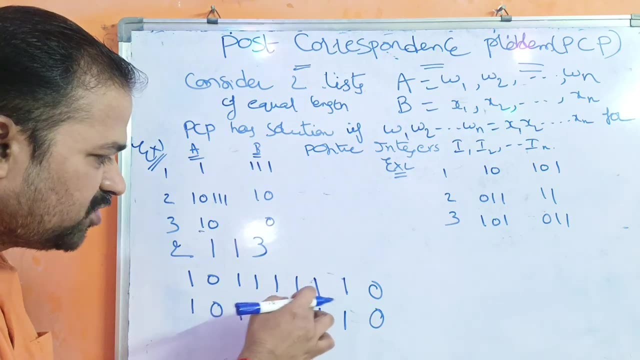 Because it is starting with 1.. So 1, 0.. So in B we have 0.. So this is the solution. If we take, if we consider the solution 1, 0, 3, 1, 1, 1, 1, 0, 1, 0, 3, 1, 1, 1, 1,. 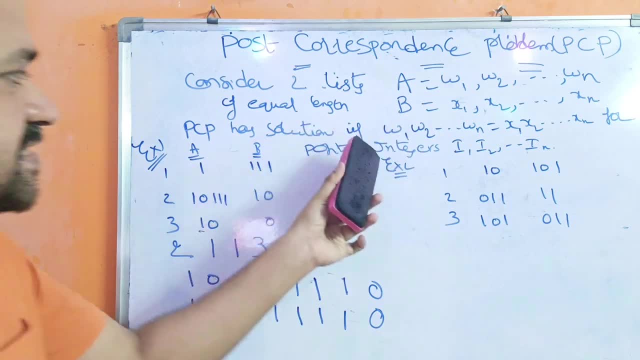 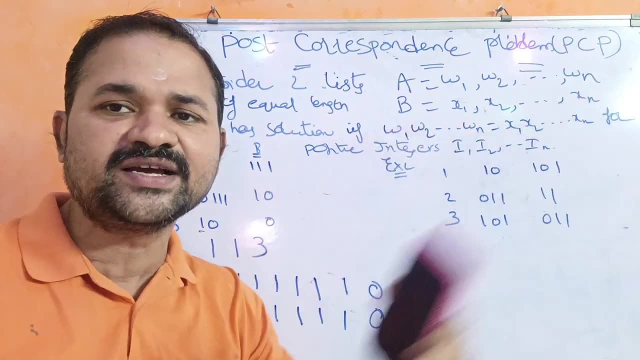 1, 0. So these two are equal. So that is the problem Here. PCP has a solution If the strings formed by concatenating the first list is equals to the strings formed by concatenating the second string. So the strings formed 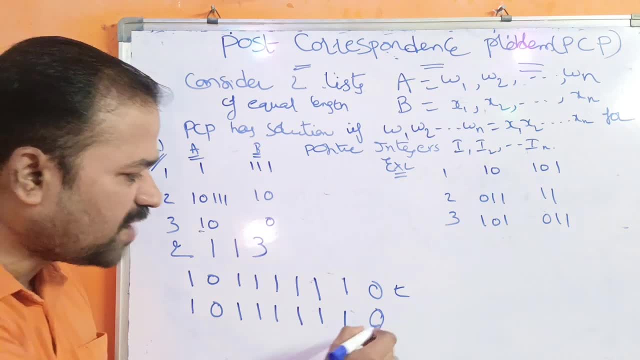 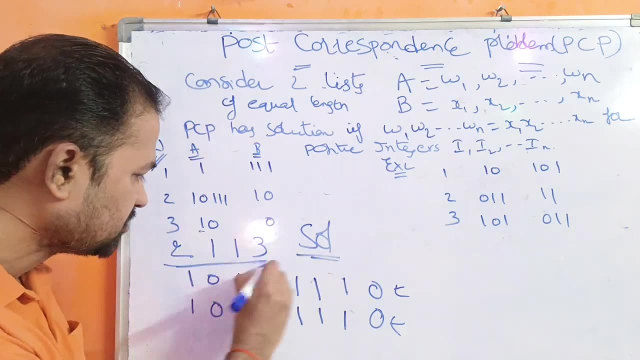 by concatenating the first string is this one. The strings formed by concatenating the second one is this one. So we can say that this problem has a solution. So this is the solution. So here we are, repeating one more than once. There is no problem, We can repeat. 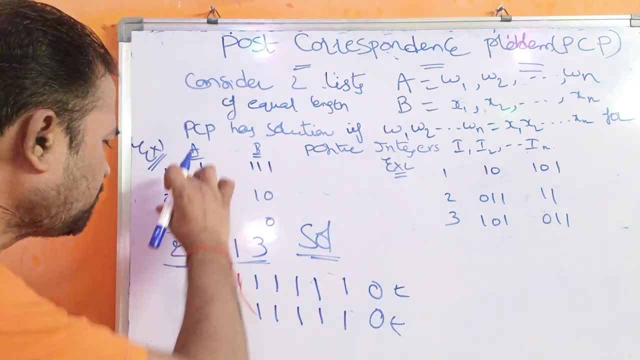 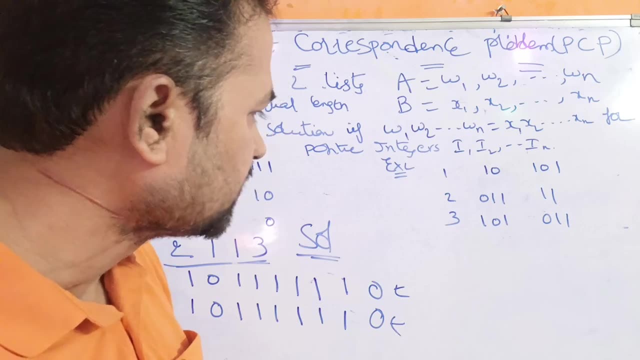 a string more than once. also, There is no problem. We have to consider all the three strings. Now let us check whether this problem has solution or not. Whether this problem has solution or not, Here we can't take 3. Why? 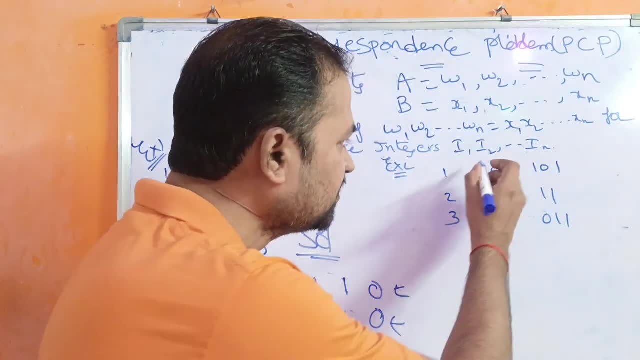 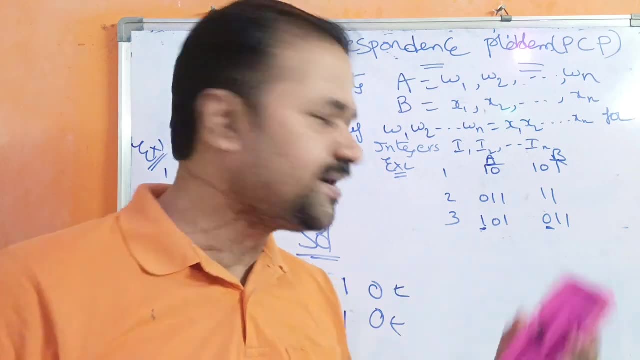 Because in 3, the first string is starting with 1.. Let this is A list, Let this is B list. It is starting with 1.. Whereas it is starting with 0. So we can't take third one. Likewise, we can't take second one also. Why? Because it is starting with 0. It is. 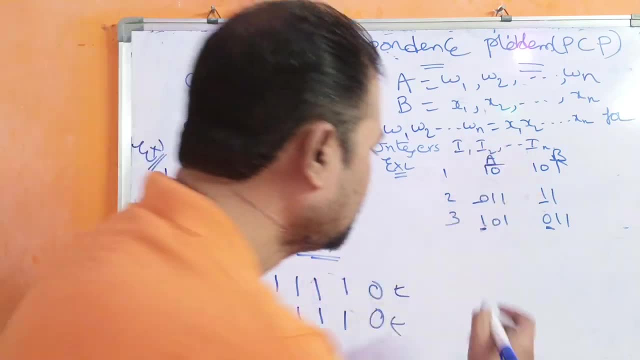 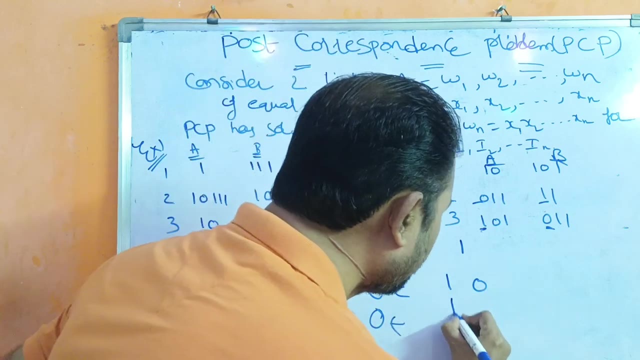 starting with 1.. So we have only one choice: That is 1.. So we have only one choice, That is 1.. So what is A string: 1, 0.. Next, what is B string: 1, 0, 1.. 1, 0, 1.. So next we have to select. 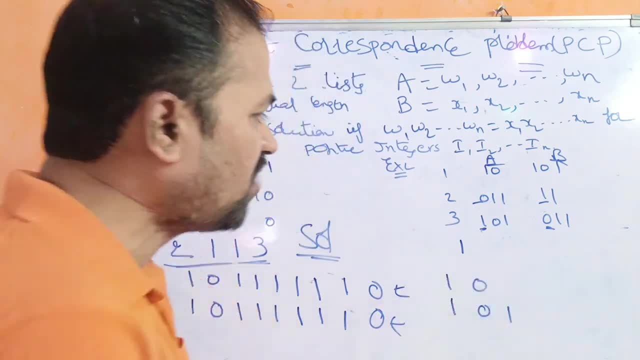 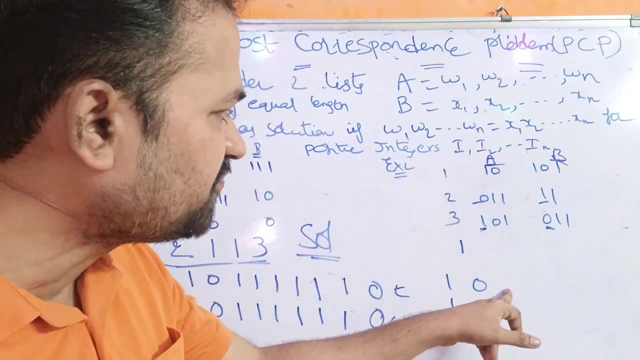 A string in such a way that it should start with 1.. So we can't take second string. So can we take the first string? Let us check here: If we take the first string, then we will get 1, 0. Why? 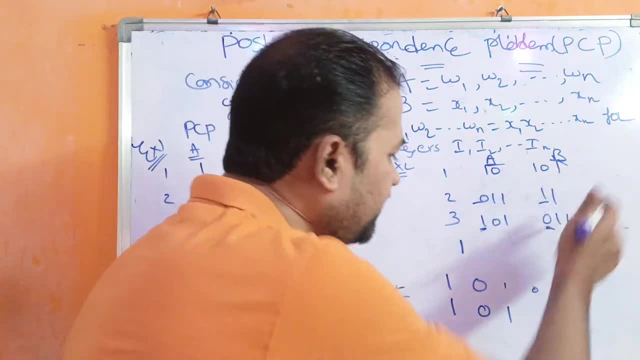 Because it is starting with 1 only, There is no problem. But here, what is B? B means 1, 0, 1.. So these two are not equal: 0, 1.. These two are not equal, So that is why we. 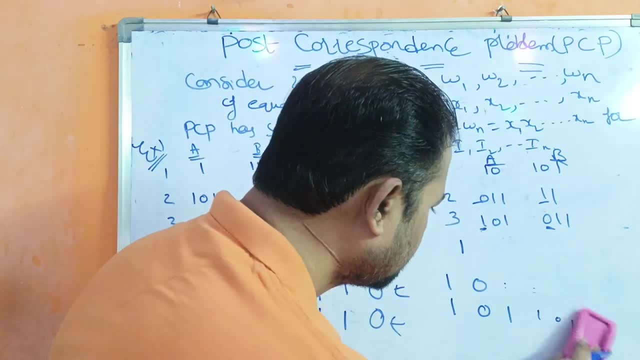 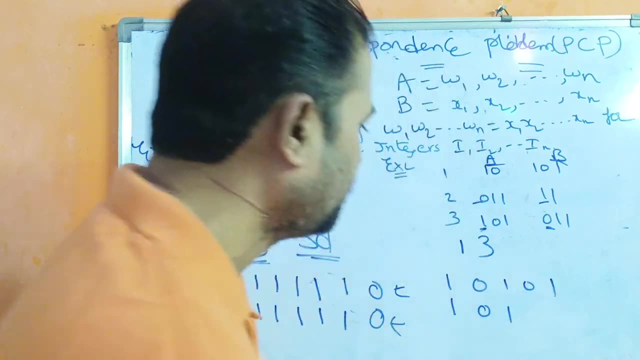 can't take 1 here. We can't take 1 here, So the other choice is 3.. So we can take 3 here. 1, 0, 1.. 1, 0, 1.. So in B we have 0, double 1.. 0, double 1.. So 1, 0, 1, 0. 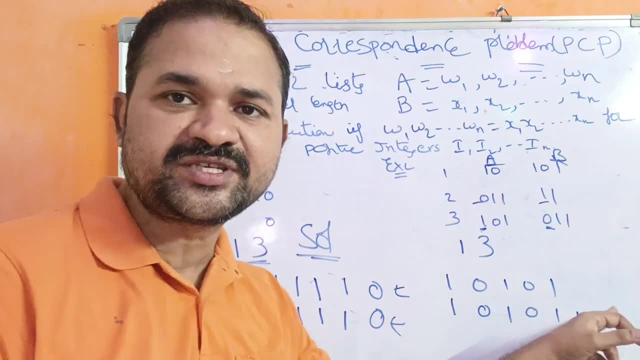 1, 0,, 1, 1.. So these two are equal. Next, we have to select S string. So we have to select S string in A such a way that it should start with 1.. So we can take either. first, 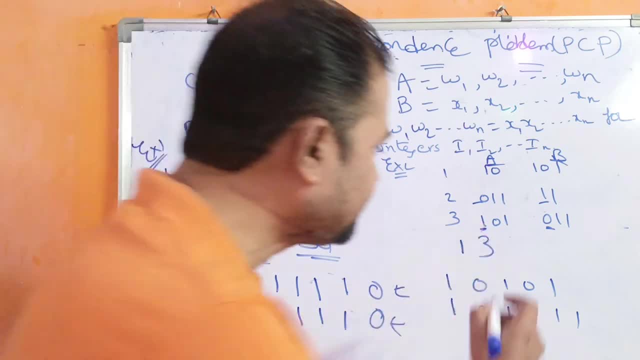 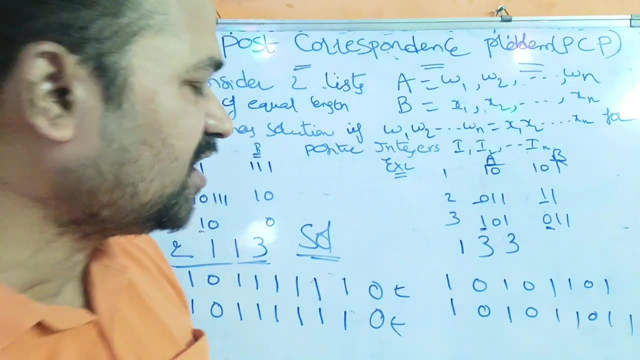 or third one, But we can't take second one, So let us take 3.. So if we take 3, then we get 1, 0, 1.. Next, 0, double 1.. So previously also here what is happening? B string contains: 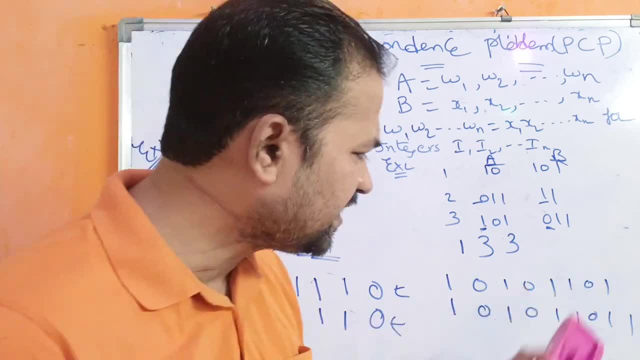 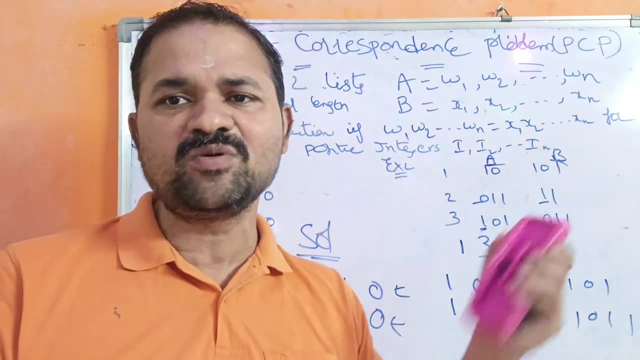 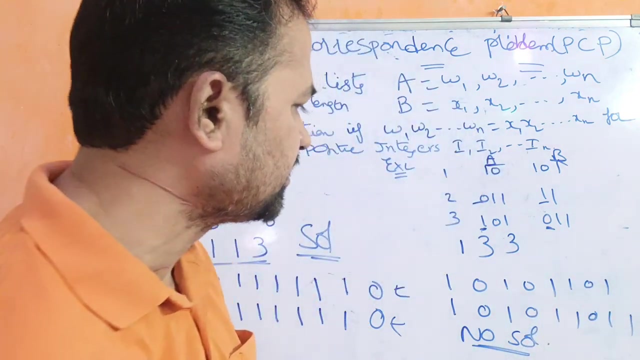 one more character than the A string. So we can say that this process will be repeated. This process will be repeated if we continue the process. So we can say that this problem has no solution. If we repeat several times. also, we don't get any solution here. So we can say that: 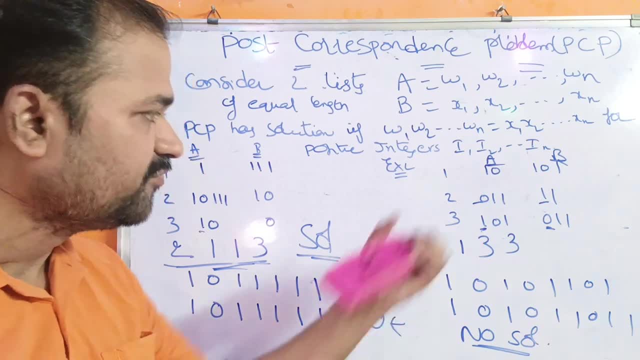 this problem has a solution. The sequence is 2, double 1,, 3,, whereas this problem has no solution. So this is about post-correspondence problem. 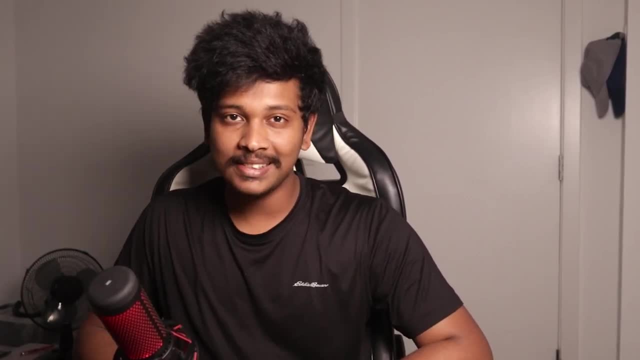 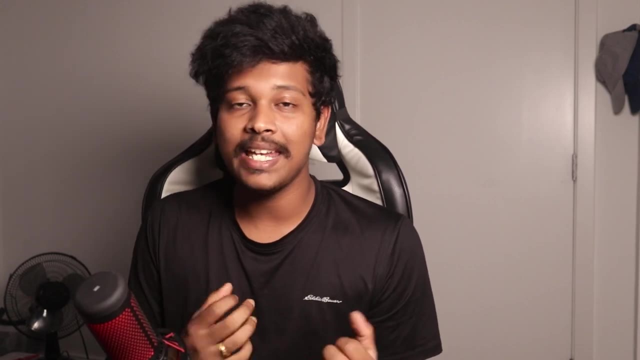 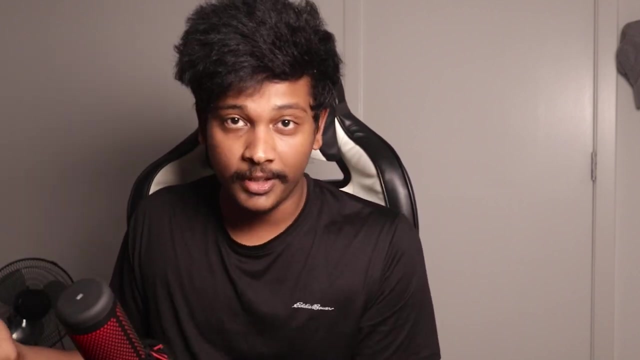 One of the most asked questions that I get from my viewers is Teja: what VPN do hackers- do real hackers- actually use to stay completely anonymous on the internet? How do they hide their real identity while browsing the internet? How do they stay anonymous In this video? 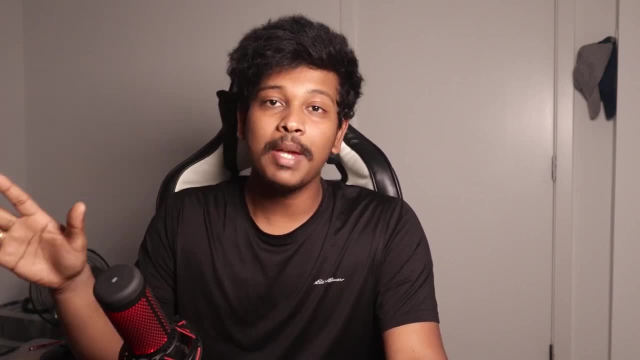 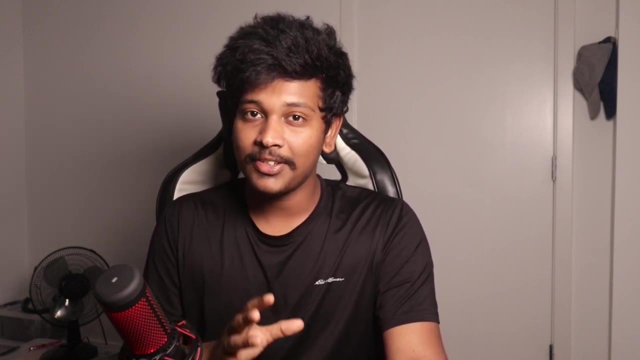 I'm going to show you how, But before getting started, let me make it very clear that the reason I'm making this video is because I believe everyone who uses internet deserves anonymity. You deserve to keep your personal identity hidden while browsing the internet.